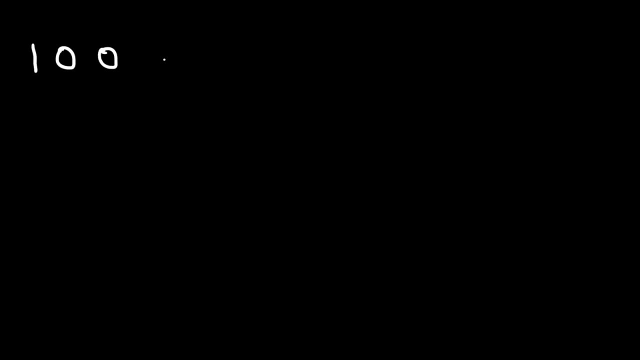 So let's say, if we have the binary number 100111.. Go ahead and convert it into an octal number. So first let's separate it into groups of three. So for the first group of three we have 100.. So everywhere there's a one we're going to. 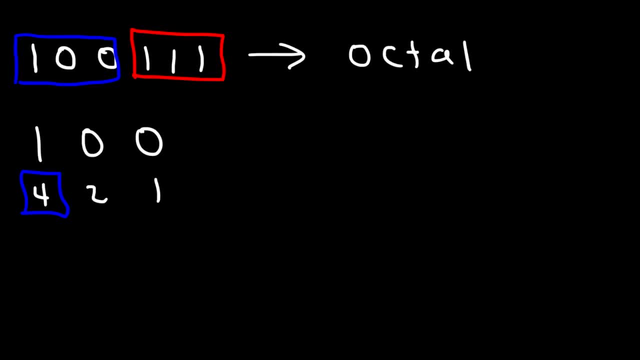 use the number that's associated with it. Binary number 100 has the equivalent of being four. Now let's do the same thing for this one. So the number is 111.. So because we have a one for each, we're going to use the four, the two and the one. 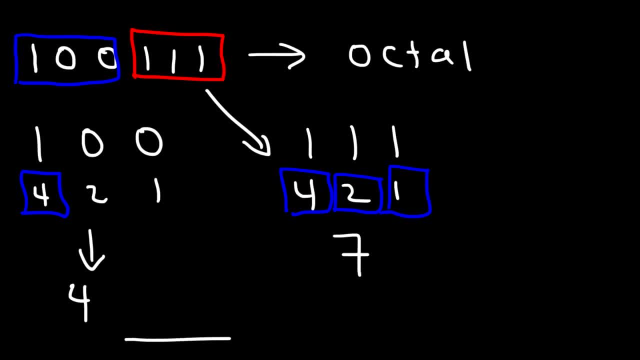 Four plus two plus one is seven. So we're going to read it this way: Our answer is 47. So it's 47 in the octal system, which is a base eight system. Now let's try a different example. So, instead of having six binary numbers, what if we have? 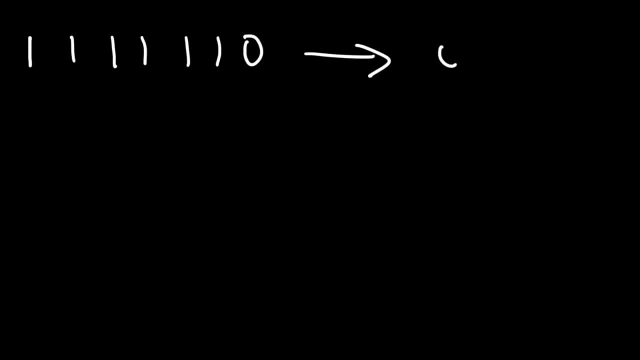 seven binary numbers. How can we convert this into an octal number? So go ahead and try it. So, once again, we're going to separate it into groups of three. So here's the first group of three and here is the second. 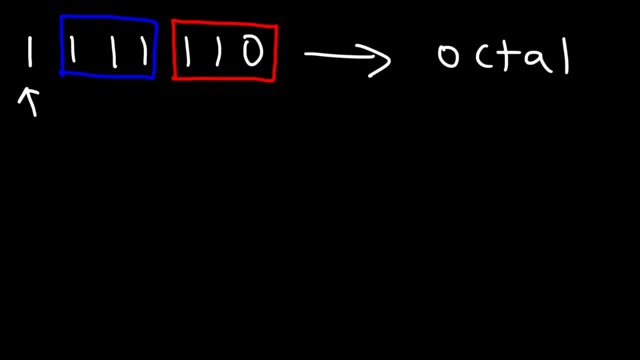 Now, because we don't have enough numbers to make another group of three, we're going to add two zeros, So it's going to be 001.. 001 is going to be 0.. 001 is going to be 0.. 002 is going to be 0.. 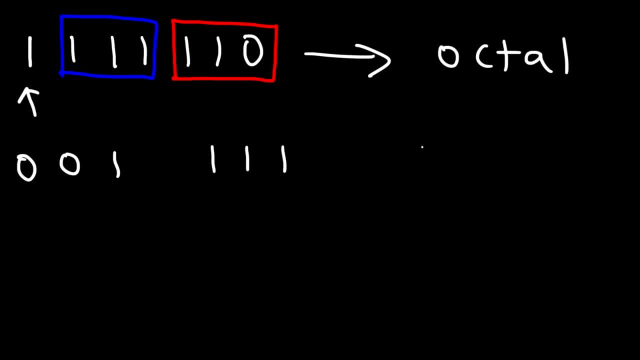 003 is going to be 0.. and then in blue, we have 1, 1, 1, and then in red, 1, 1, 0.. So let's start with this example. So we have 4, 2, 1, and so this will have a value of 1.. 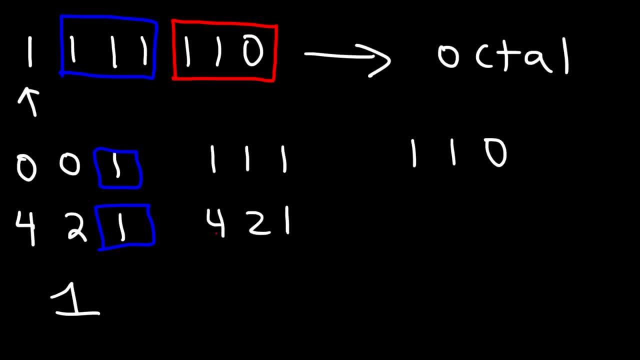 For the next one, it's 1, 1, 1, so we need to add up each number. We have a 1 associated with the 4, the 2 and the 1.. 4 plus 2 plus 1 is 7, and for the next one we have a 1 in front of the 4 and in front. 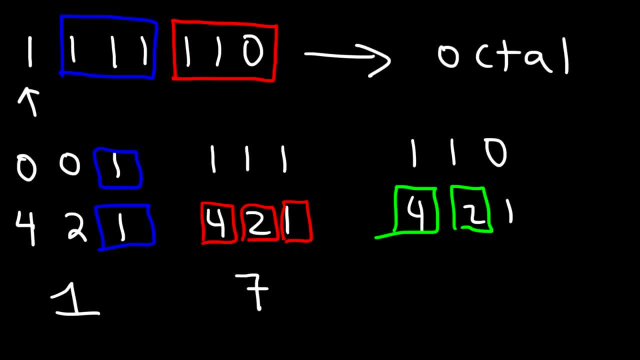 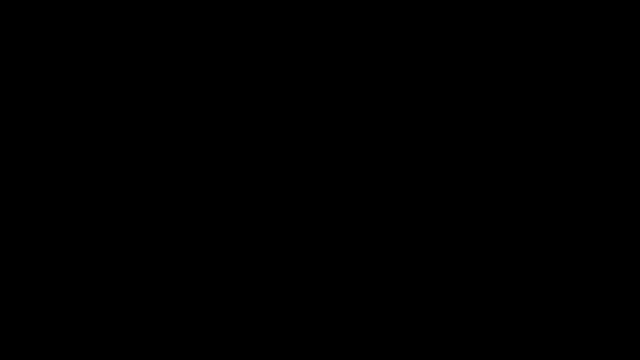 of the 2, so we're only going to add 4 plus 2, which is 6, and so you can see the answer: it's 176, and so that's it for this problem. Now, for the sake of practice, let's do one more example.